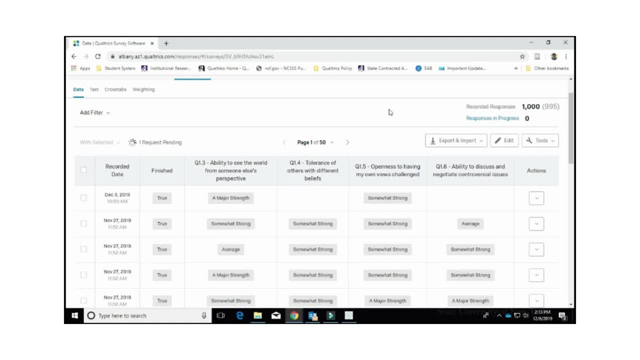 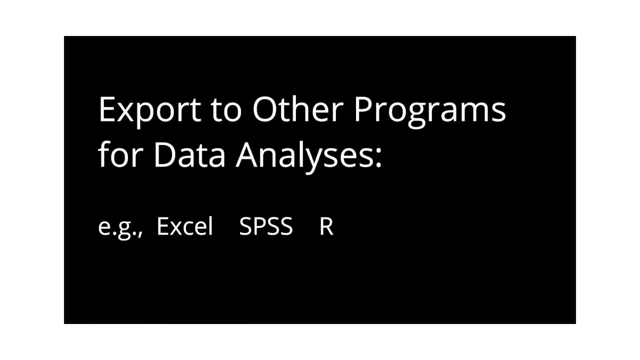 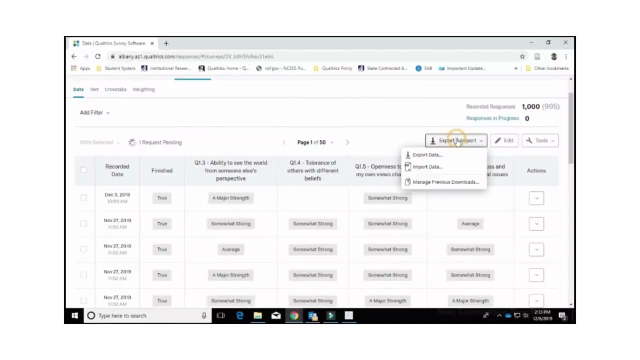 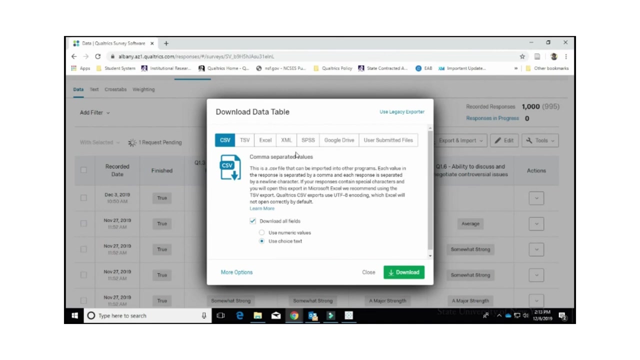 In terms of data analysis. there are two options here. You can either export the data from Qualtrics and conduct analyses in other programs such as Microsoft Excel, SPSS and R, or perform data analysis right in Qualtrics. To analyze data in other programs, select the Export Data button from the Export and Import dropdown. 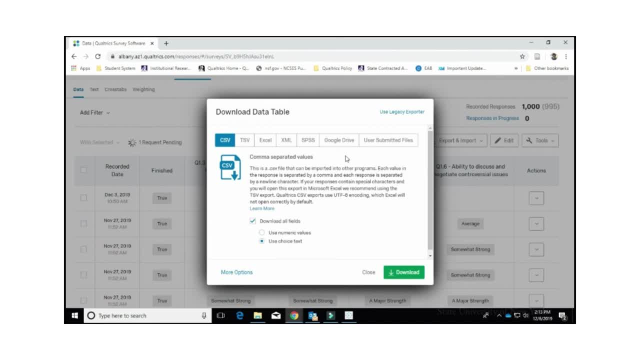 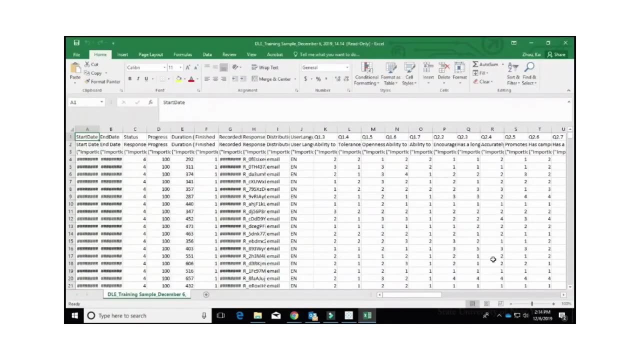 Then you can choose a file format. CSV and SPSS are the two most commonly used formats for data analysis. CSV provides an Excel-compatible file. Click Download and obtain your file after the download process is completed. Here's a screenshot of what an Excel data file looks like. 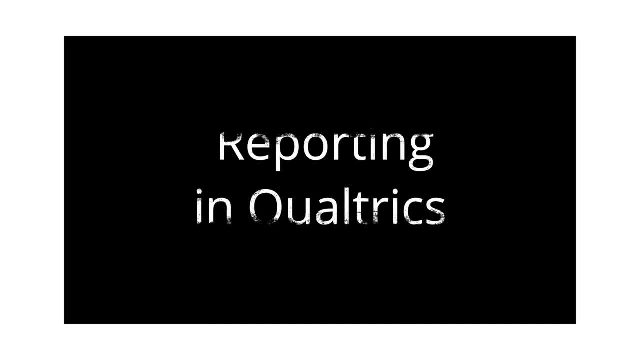 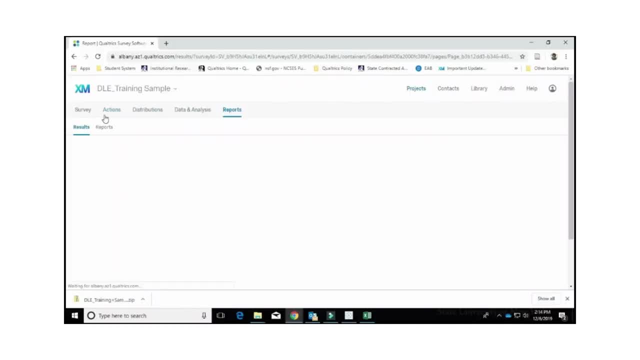 In this tutorial we would like to show you how to perform simple analyses and produce descriptive table and graph reports directly in Qualtrics. Go to Reports In the Results section. Qualtrics generates a default report that provides information of the choice frequencies for each question. 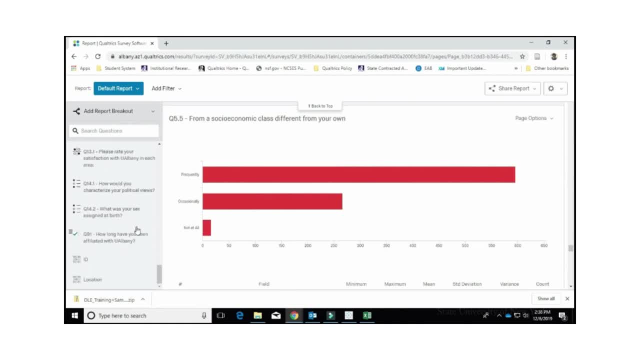 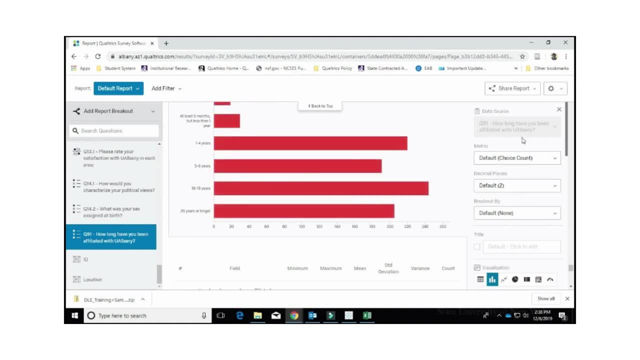 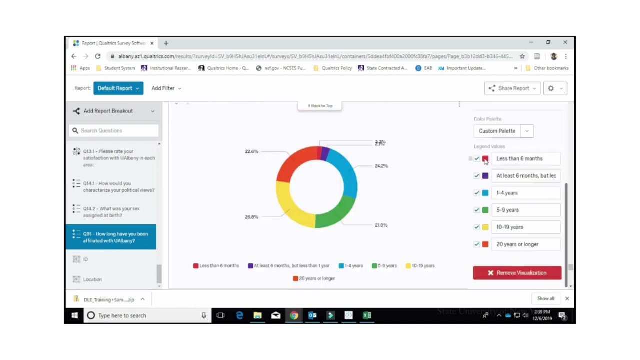 Click any visualization to open its editing pane. You can customize visualizations quickly by picking from the editing pane. You're free to change color schemes and chart or table types. For example, you may want to change the metric from choice count to percentage, change a bar chart to a pie chart and change the color red to orange. 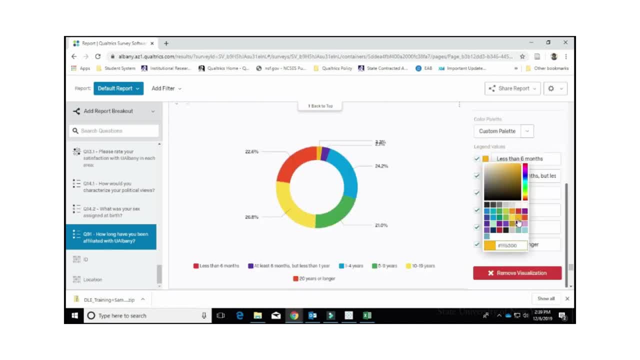 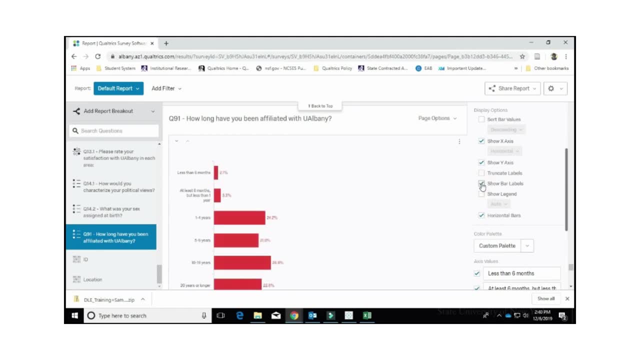 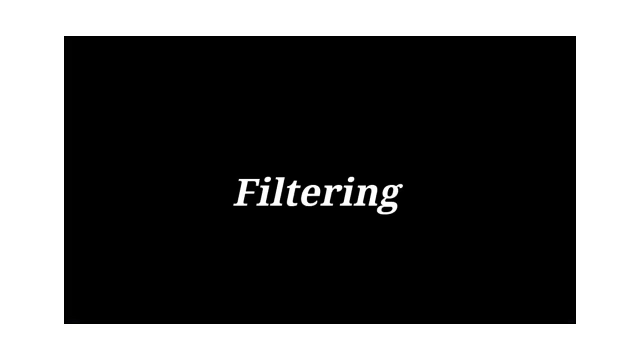 You may also display data by checking the Show Bar Labels box. You can also break out your results in Qualtrics. You can also break out your results by group, for example by gender. The filtering option can help you screen out the data that you don't need at the moment. 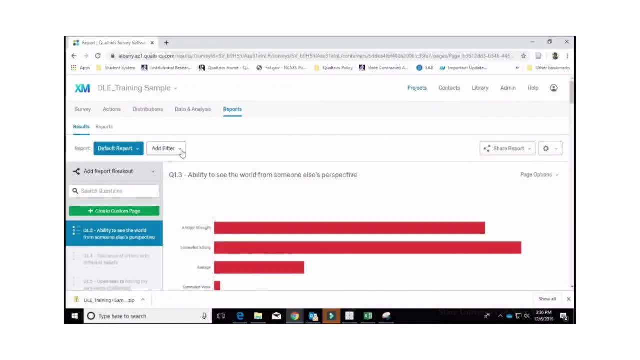 You can create your conditional statements by clicking Add Filter. For example, you might want to focus on female participants. Select the demographic question 14.2,. select a choice, select operator and pick an operator. Here we choose is and pick your operand. 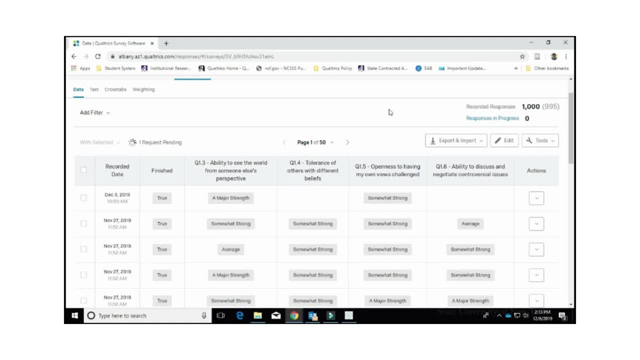 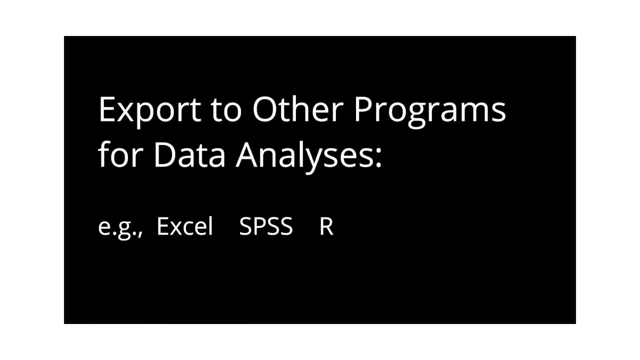 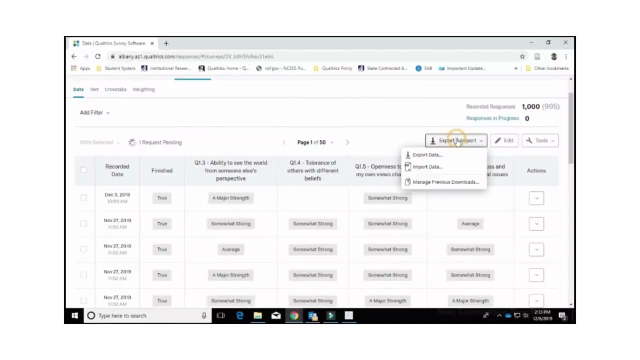 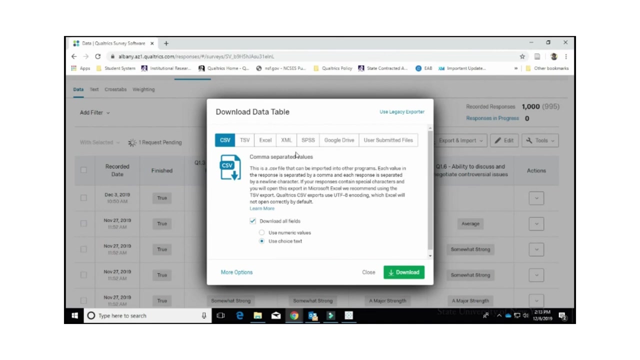 In terms of data analysis. there are two options here. You can either export the data from Qualtrics and conduct analyses in other programs such as Microsoft Excel, SPSS and R, or perform data analysis right in Qualtrics. To analyze data in other programs, select the Export Data button from the Export and Import dropdown. 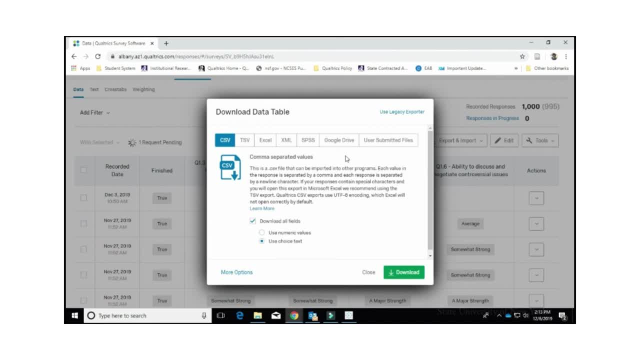 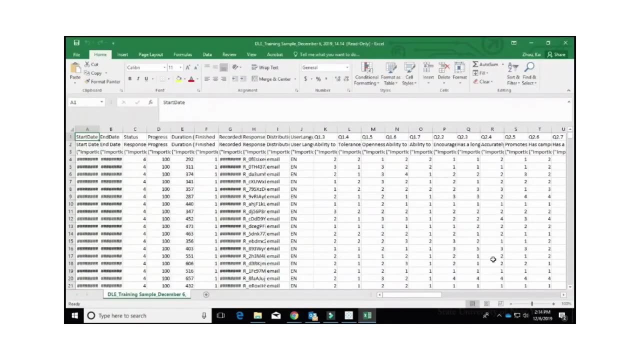 Then you can choose a file format. CSV and SPSS are the two most commonly used formats for data analysis. CSV provides an Excel-compatible file. Click Download and obtain your file after the download process is completed. Here's a screenshot of what an Excel data file looks like. 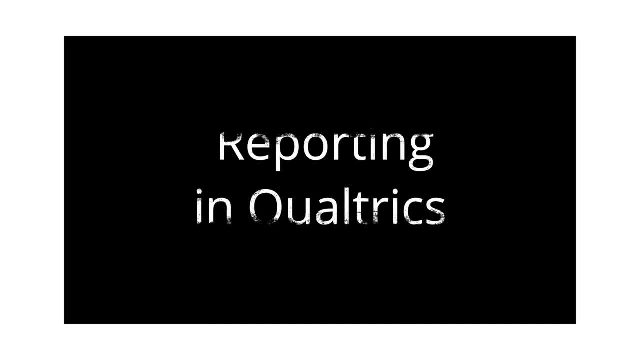 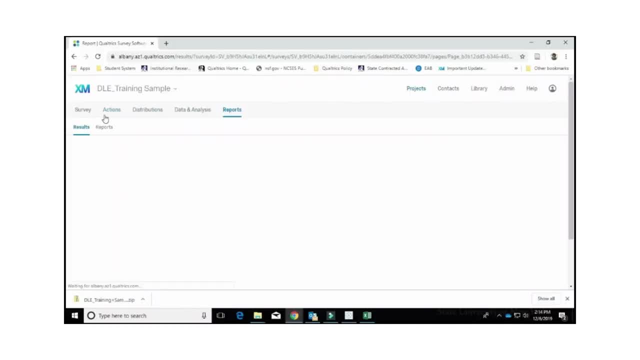 In this tutorial we would like to show you how to perform simple analyses and produce descriptive table and graph reports directly in Qualtrics. Go to Reports In the Results section. Qualtrics generates a default report that provides information of the choice frequencies for each question. 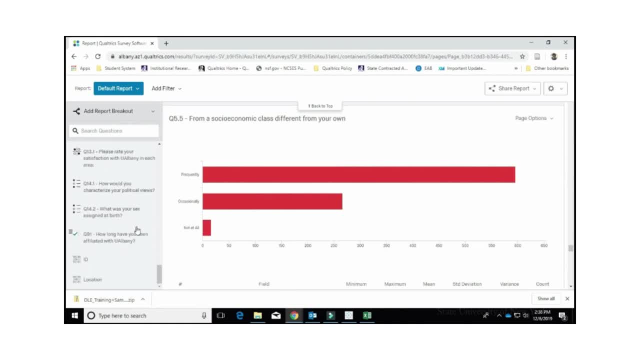 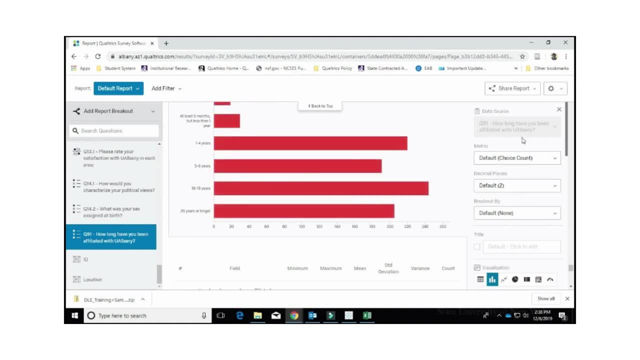 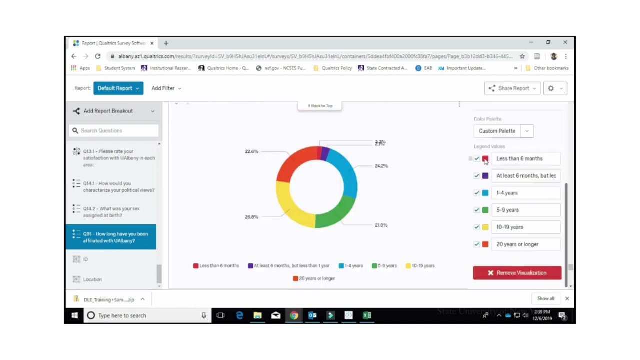 Click any visualization to open its editing pane. You can customize visualizations quickly by picking from the editing pane. You're free to change color schemes and chart or table types. For example, you may want to change the metric from choice count to percentage, change a bar chart to a pie chart and change the color red to orange. 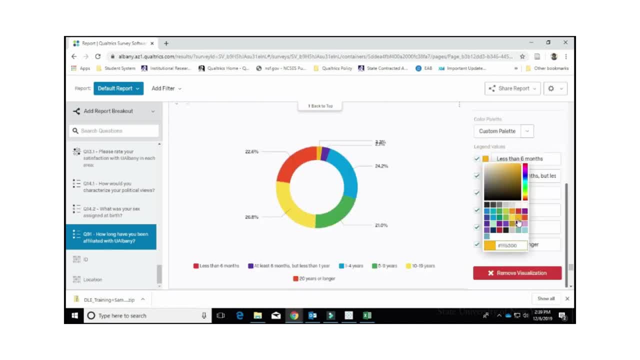 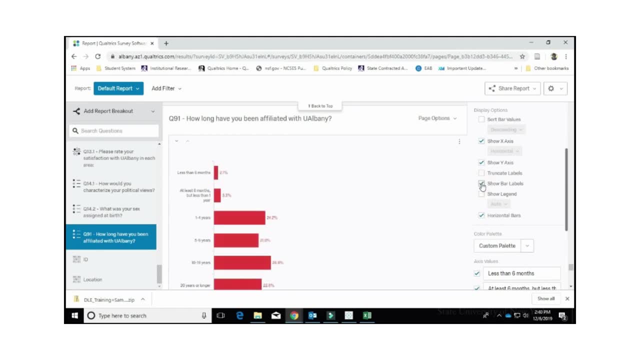 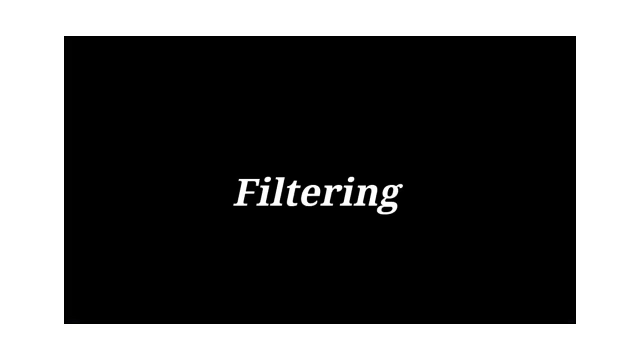 You may also display data by checking the Show Bar Labels box. You can also break out your results in Qualtrics. You can also break out your results by group, for example by gender. The filtering option can help you screen out the data that you don't need at the moment. 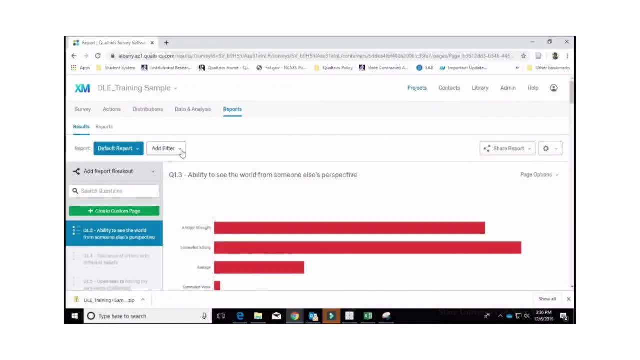 You can create your conditional statements by clicking Add Filter. For example, you might want to focus on female participants. Select the demographic question 14.2,. select a choice, select operator and pick an operator. Here we choose is and pick your operand. 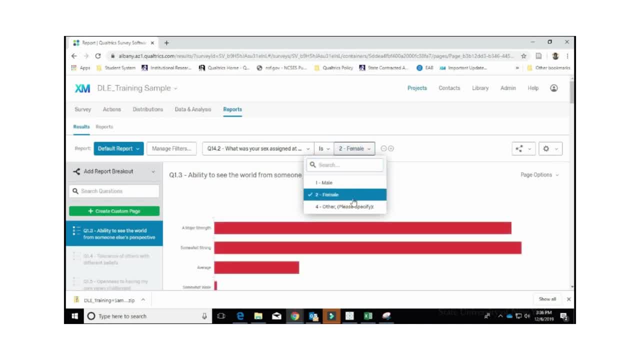 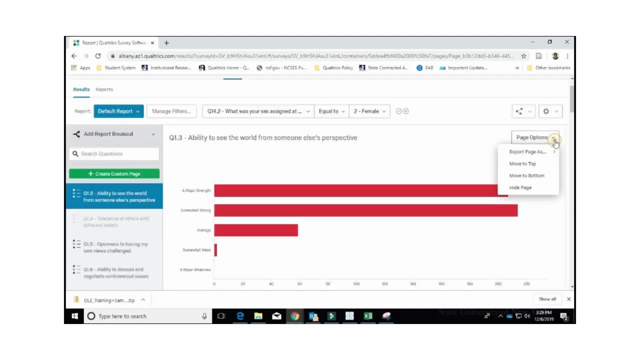 The value. here we choose 2, female, and apply it to the conditional statement. Now the filter we just created changed the visualizations. You can export a single visualization by selecting the question item. Choose Page Options, Export Page As and then select the desired format. 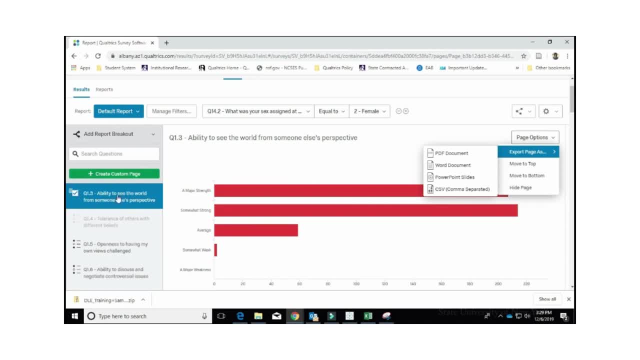 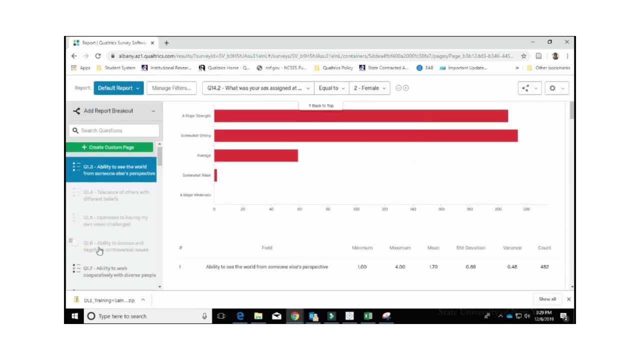 If you don't want to show all of the questions on the report. instead you just want to show part of the survey results. you can hide questions that you don't want to display in the report. Go to the left on the pane and uncheck the box for those unwanted questions. 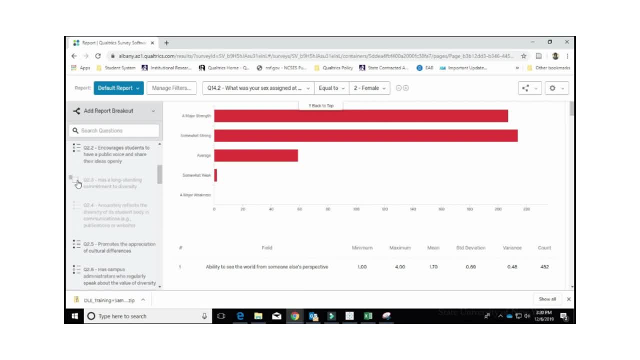 If you don't like some of the displays on the report- for example, you just want to show the bar chart, not a statistics description table- you can click the three dots on the top right and then select Remove Visualization. If you want to write a short paragraph to describe the results, 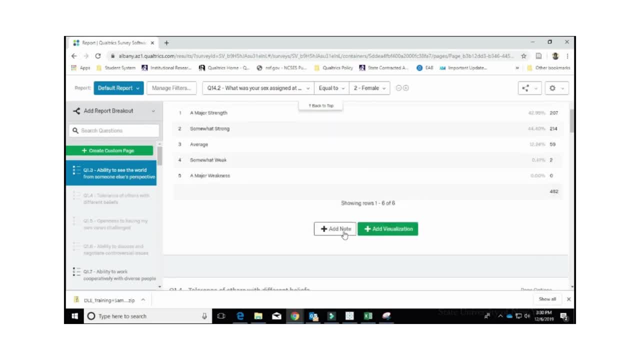 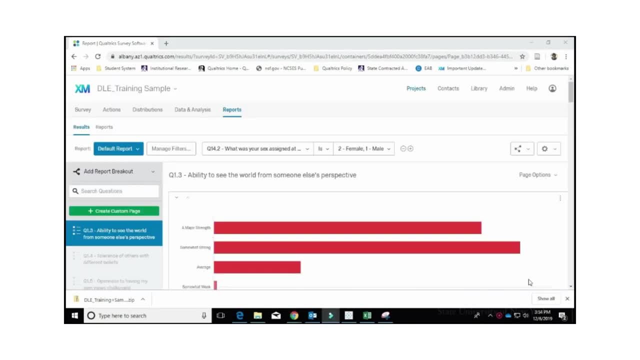 and help stakeholders interpret the data. you can click Add Note and type in your descriptions After you modify your report. you can share a results report. Go to Share Report. There are many ways to share your report, such as generating a digital copy in a PDF, Word or PowerPoint format. 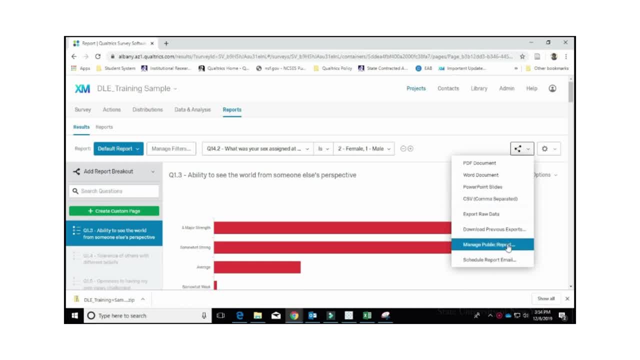 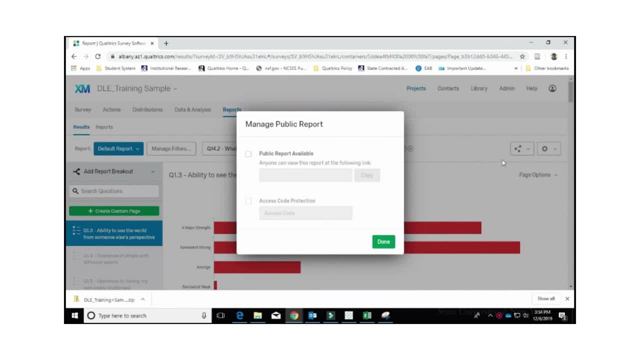 Or you can share your report with a friend or with a web link by selecting Manage Public Report. A public report is dynamic, interactive and updates in real time. Any changes to the Qualtrics report are posted immediately and can be viewed via the link. 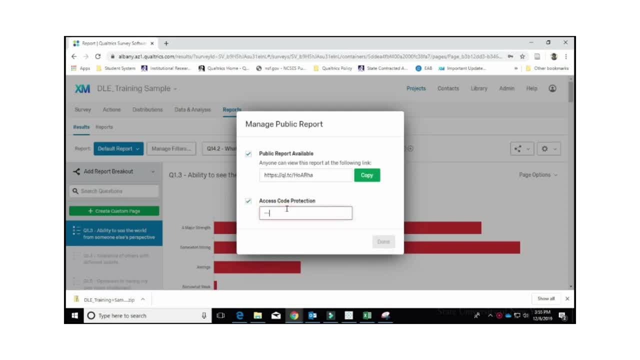 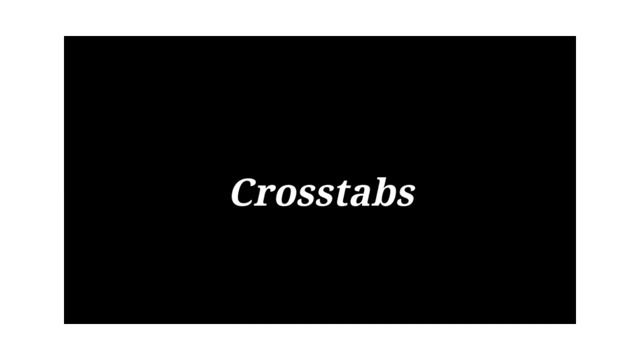 Choose Public Report Available. You can add an access code which allows only a certain group of people to view the report. Copy the link and click Done. If you would like to conduct multivariate analyses that are beyond describing frequencies and row percentages, you can use the Cross Tabs page under Data and Analyses. 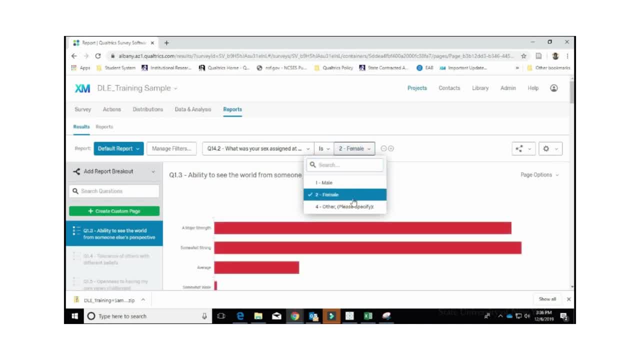 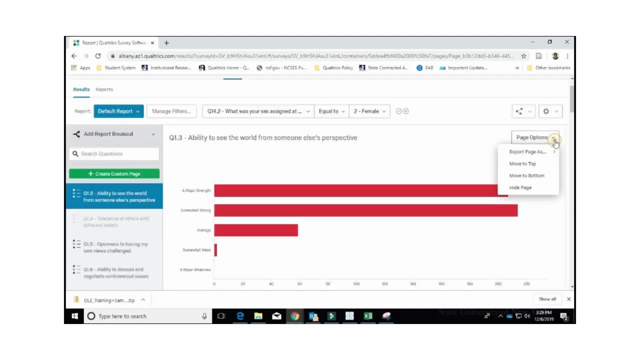 The value. here we choose 2, female, and apply it to the conditional statement. Now the filter we just created changed the visualizations. You can export a single visualization by selecting the question item. Choose Page Options, Export Page As and then select the desired format. 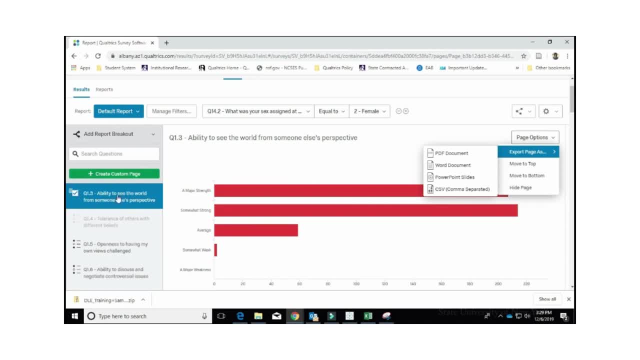 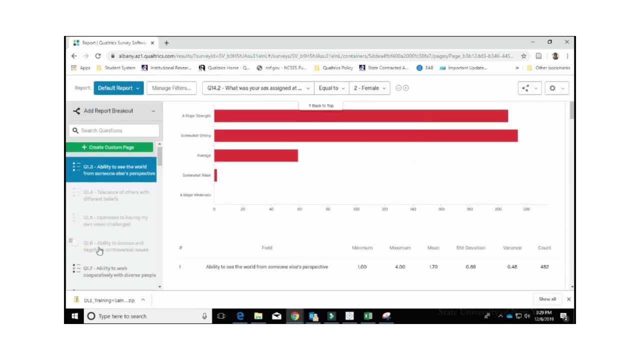 If you don't want to show all of the questions on the report. instead you just want to show part of the survey results. you can hide questions that you don't want to display in the report. Go to the left on the pane and uncheck the box for those unwanted questions. 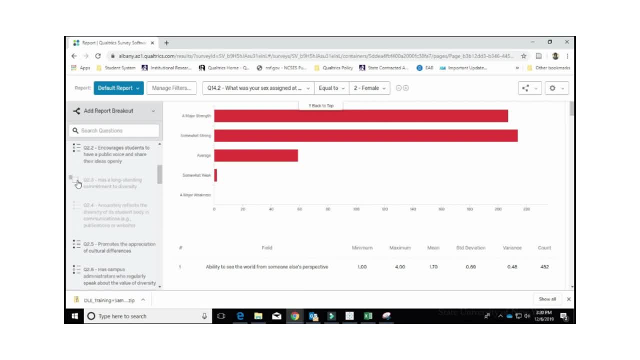 If you don't like some of the displays on the report- for example, you just want to show the bar chart, not a statistics description table- you can click the three dots on the top right and then select Remove Visualization. If you want to write a short paragraph to describe the results, 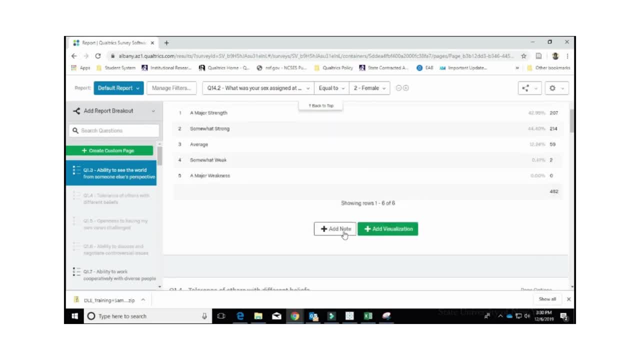 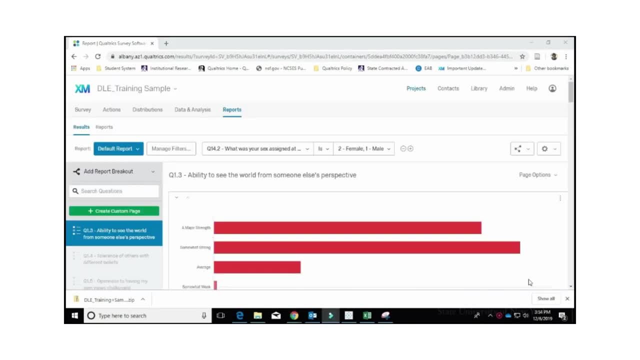 and help stakeholders interpret the data. you can click Add Note and type in your descriptions After you modify your report. you can share a results report. Go to Share Report. There are many ways to share your report, such as generating a digital copy in a PDF, Word or PowerPoint format. 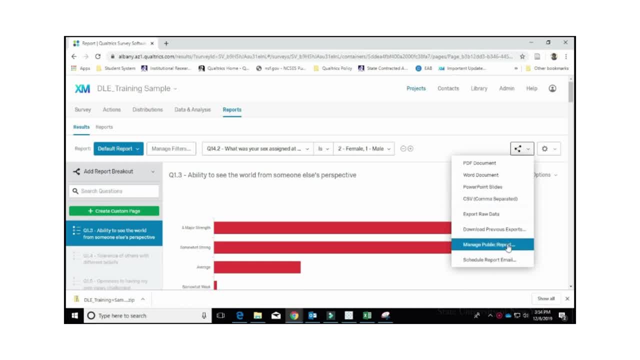 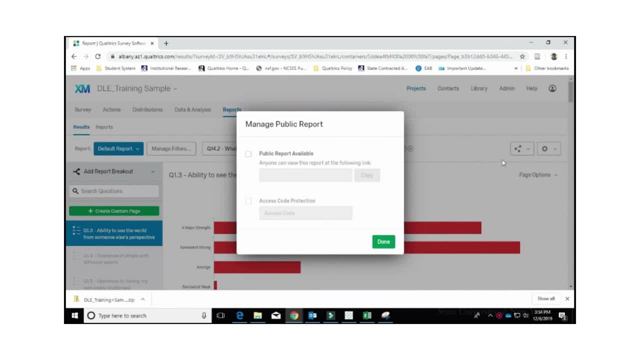 Or you can share your report with a friend or with a web link by selecting Manage Public Report. A public report is dynamic, interactive and updates in real time. Any changes to the Qualtrics report are posted immediately and can be viewed via the link. 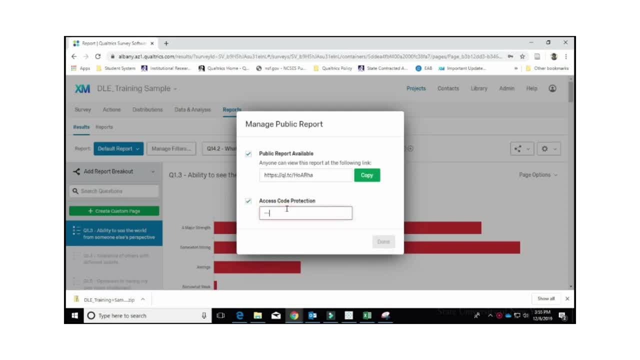 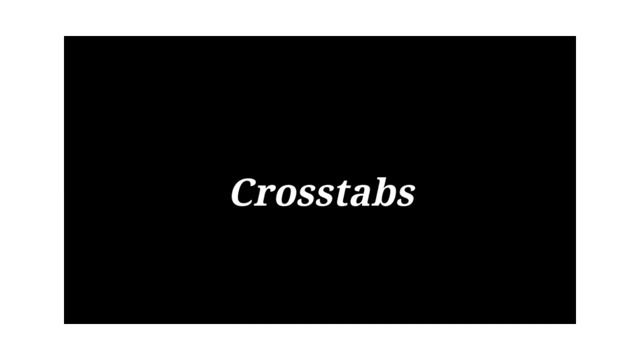 Choose Public Report Available. You can add an access code which allows only a certain group of people to view the report. Copy the link and click Done. If you would like to conduct multivariate analyses that are beyond describing frequencies and row percentages, you can use the Cross Tabs page under Data and Analyses. 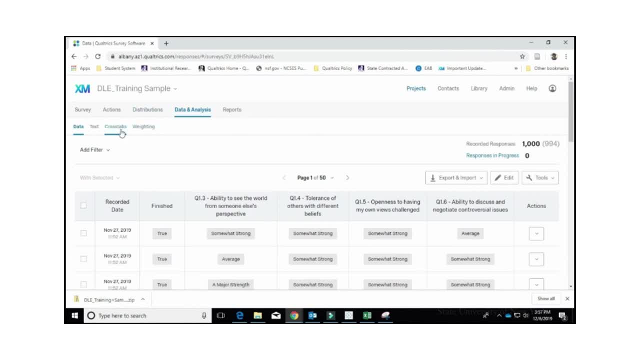 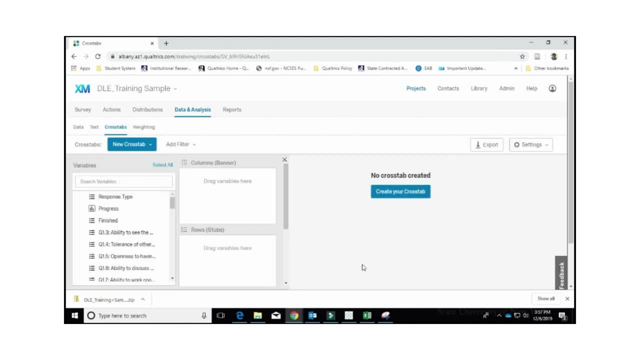 Again. take the Diversity Climate Survey as an example. You may want to perform chi-squared analyses to see whether there is a relationship between years of affiliation with the institution and their self-reported ability to see the world from someone else's perspective. You can drag Q91,. 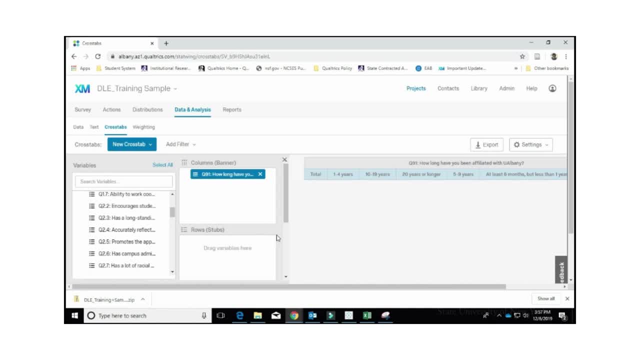 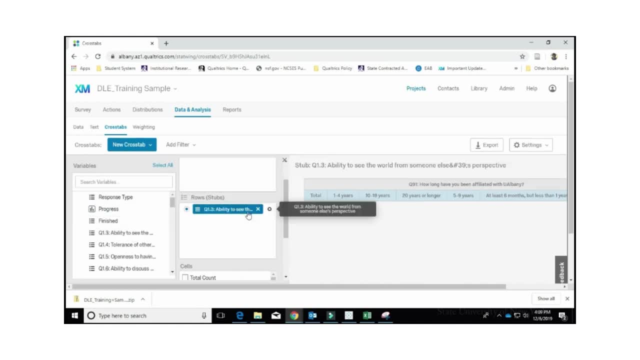 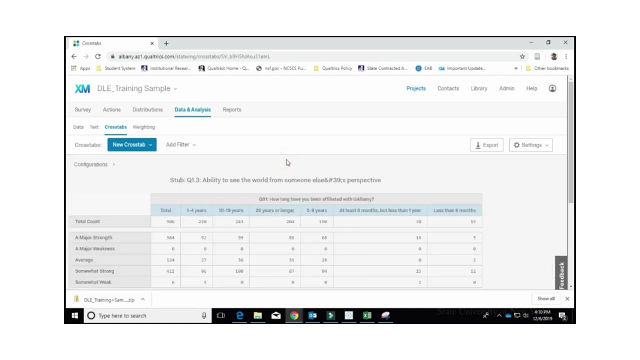 how long have you been affiliated with the institution? into columns in the variable Q1.3, ability to see the world from someone else's perspective. into rows. Then select Total Count Counts and Column Percentages. The Cross Tab analysis shows that 220 individuals. 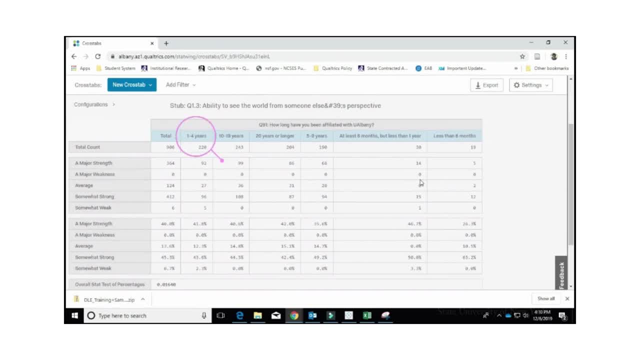 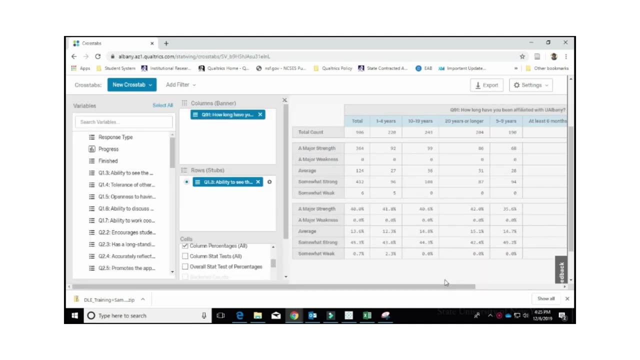 who have been affiliated with the institution between 1 to 4 years answered question 1.3.. 41.8% reported that they had a major strength in the ability to see the world from someone else's perspective. Then we can also perform a chi-squared test in Qualtrics. 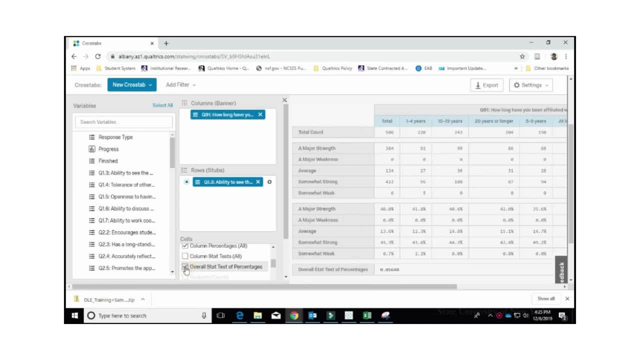 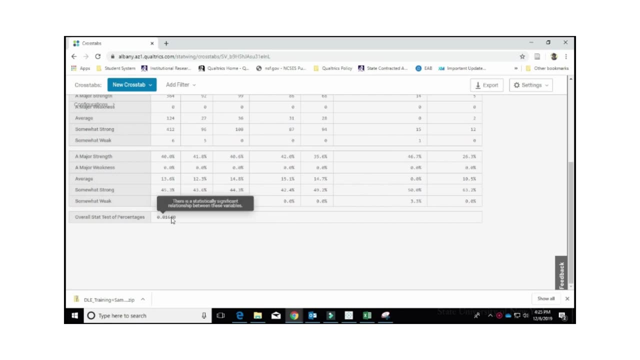 to test the significance of the group differences, Select Overall Stat Test of Percentages. A p-value is calculated in Qualtrics. The p-value here shows that the self-ratings on the ability to see the world from someone else's perspective are, on average, statistically different for the affiliation year group. 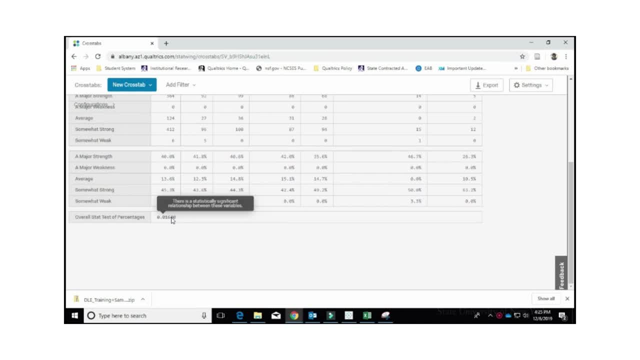 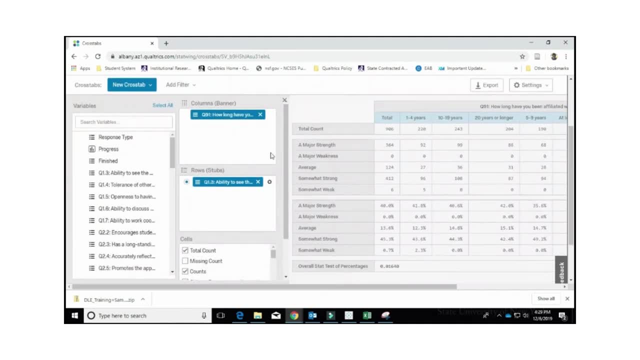 at a significance level of p less than .05.. You can also create nesting columns to have one set of variables splitting another. For example, we would like to see a breakdown of gender nested under affiliation year, Instead of having male and female in six affiliation year categories separately. 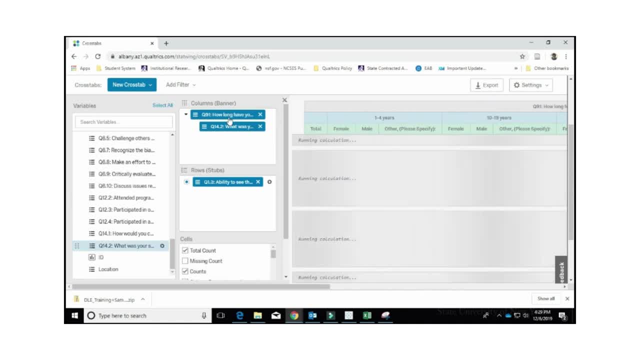 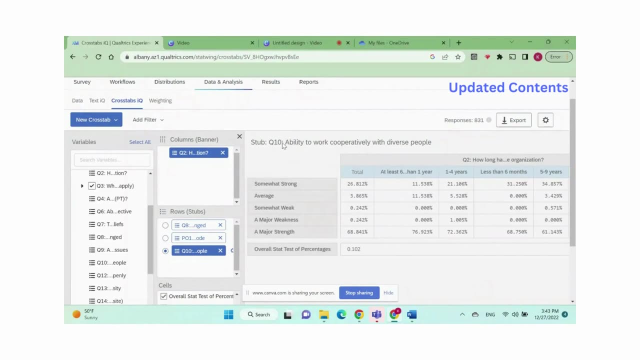 you get 12 aggregated columns. We just need to drag the variable Q14.2- Sex Identification- under the variable Q91- Year of Affiliation, Then the results are updated. One thing should be noted is that in the Cross Tab the variables are not always presented in the correct order. 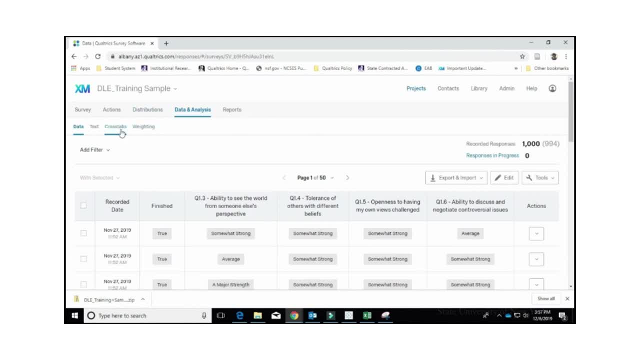 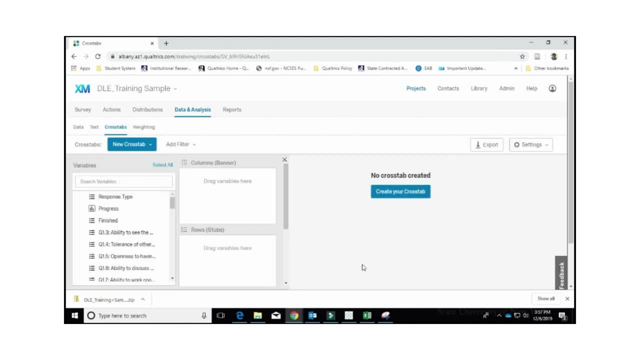 Again. take the Diversity Climate Survey as an example. You may want to perform chi-squared analyses to see whether there is a relationship between years of affiliation with the institution and their self-reported ability to see the world from someone else's perspective. You can drag Q91,. 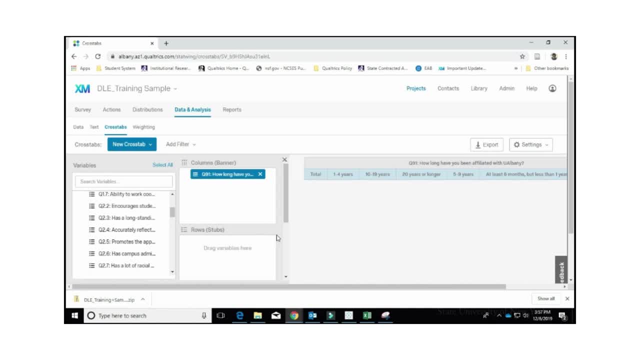 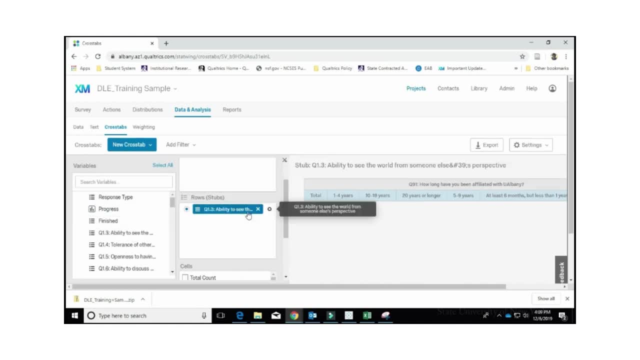 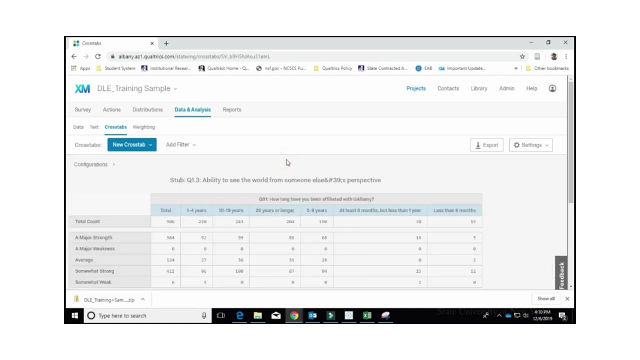 how long have you been affiliated with the institution? into columns in the variable Q1.3, ability to see the world from someone else's perspective. into rows. Then select Total Count Counts and Column Percentages. The Cross Tab analysis shows that 220 individuals. 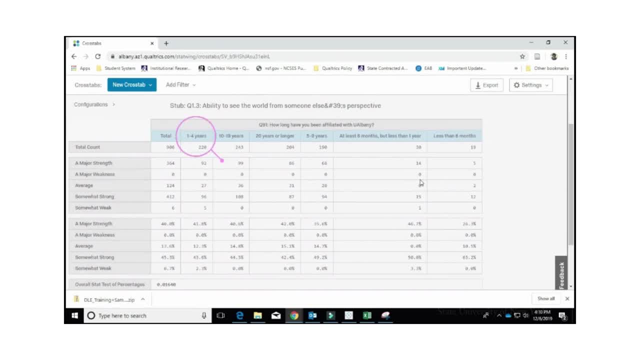 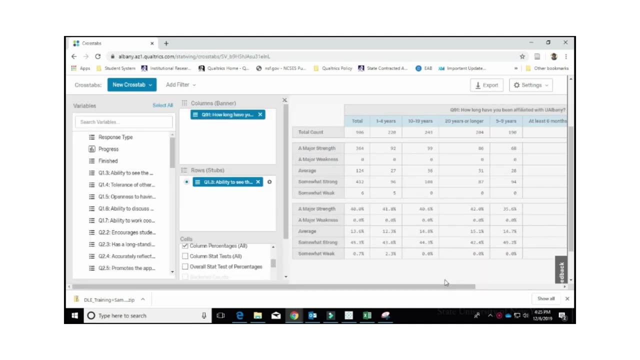 who have been affiliated with the institution between one to four years answered question 1.3.. 41.8% reported that they had a major strength in the ability to see the world from someone else's perspective. Then we can also perform a chi-squared test in Qualtrics. 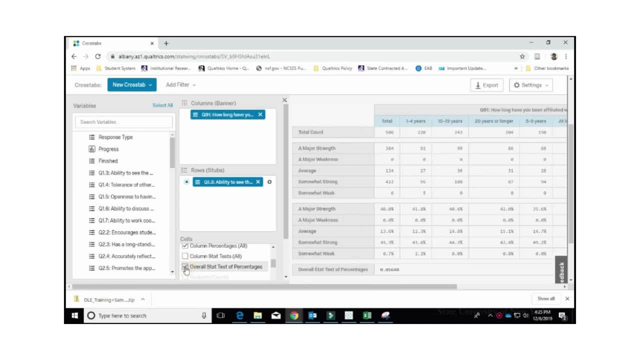 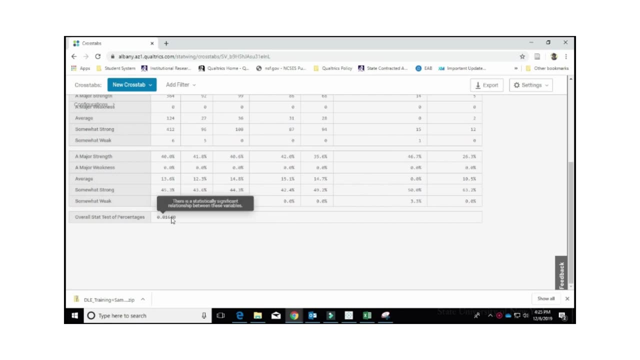 to test the significance of the group differences, Select Overall Stat Test of Percentages. A p-value is calculated in Qualtrics. The p-value here shows that the self-ratings on the ability to see the world from someone else's perspective are, on average, statistically different for the affiliation year group. 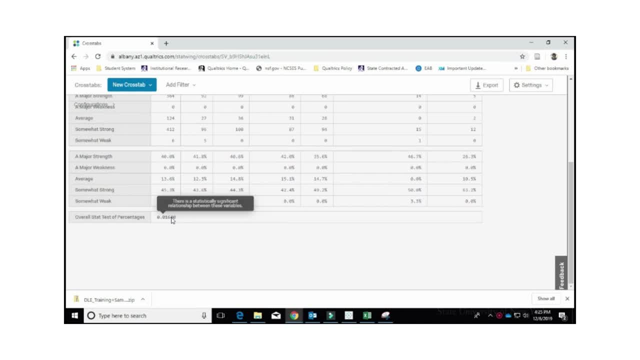 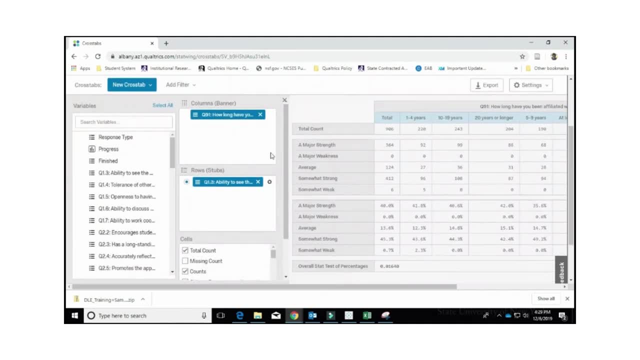 at a significance level of p less than .05.. You can also create nesting columns to have one set of variables splitting another. For example, we would like to see a breakdown of gender nested under affiliation year, Instead of having male and female in six affiliation year categories separately. 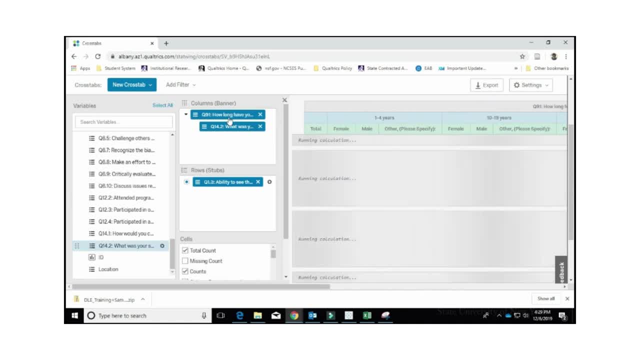 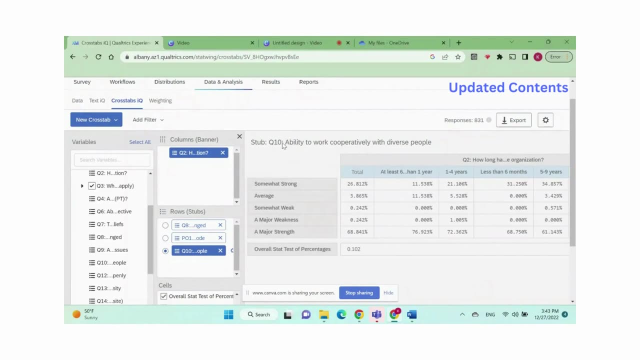 you get 12 aggregated columns. We just need to drag the variable Q14.2- Sex Identification- under the variable Q91- Year of Affiliation, Then the results are updated. One thing should be noted is that in the Cross Tab the variables are not always presented in the correct order. 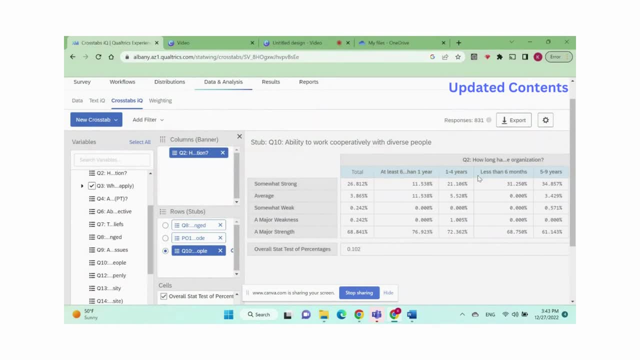 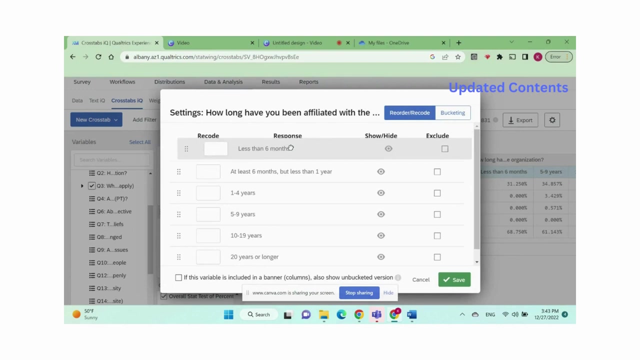 For example, in Question 2, less than six months option should be presented first before the choice at least six months, but less than one year. To reorder the choices, we click the setting icon of the variable in the banner window. Choose the choice you want to move and drag it to the right place. 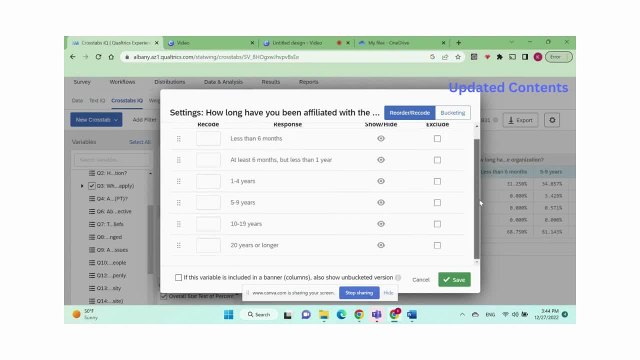 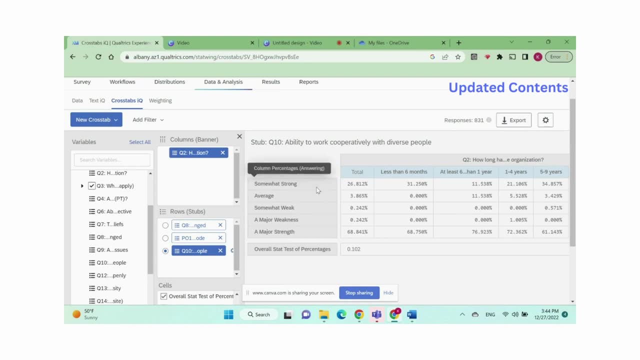 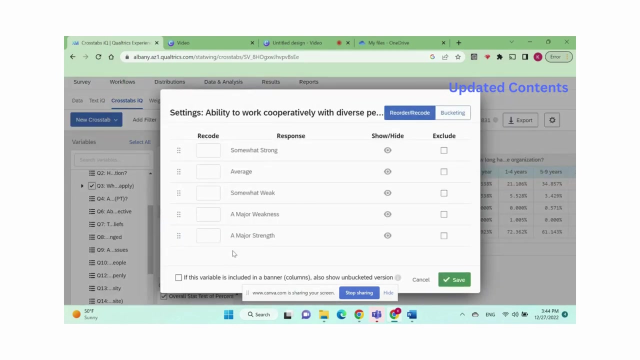 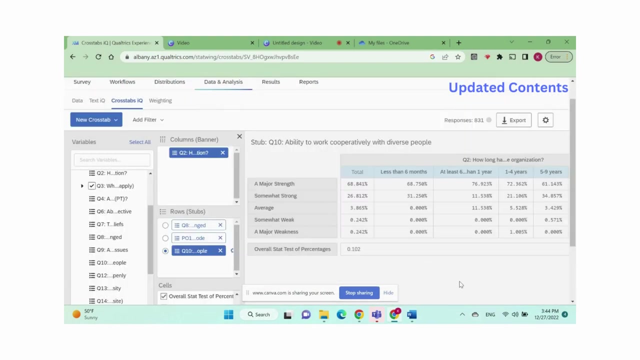 Then click Save. Same issue is found with the scale points in the rows. We click the setting icon of the scale variable in the stubs window, Drag the selected scale point to the correct place, Then save. Sometimes we may want to group some scale points together. 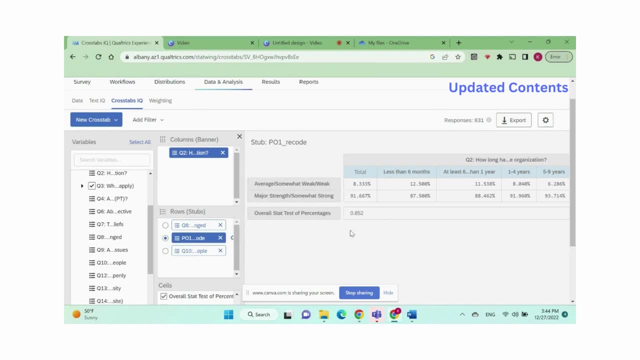 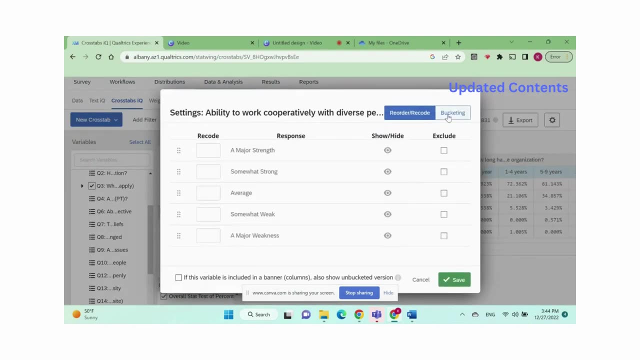 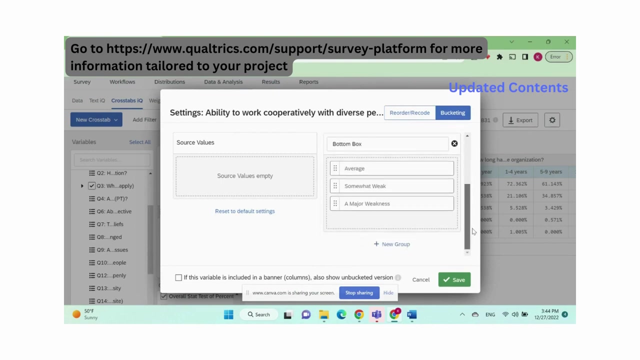 to get more meaningful analysis. For example, we can combine major strength in somewhat strong and major weakness in somewhat weak Together. by using the bucketing feature in Qualtrics We can varying the weight and size of the scale. We can also use the small scale for bathroom height. 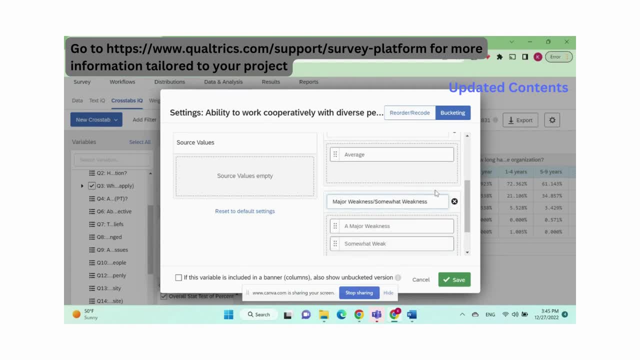 That may be the most personable solution To configure the scale. we click when it's at the bottom of the screen. As the scale increases, the scale will be raised or not. Here again, when we click the scale, the scale will be raised or not. 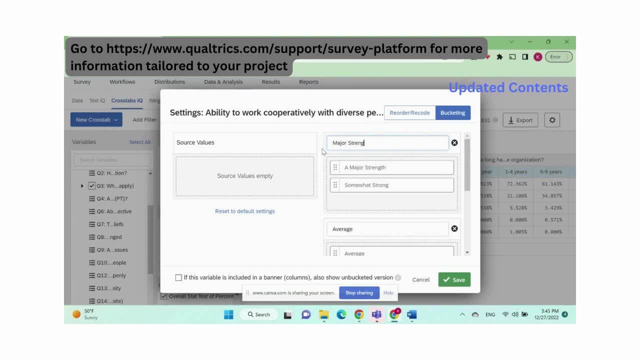 And when we click next, the scale will be raised. When we click next, the scale will be raised or not. This way, we can generate more interesting analysis. Now we can see that the scale is not the same as the background size. 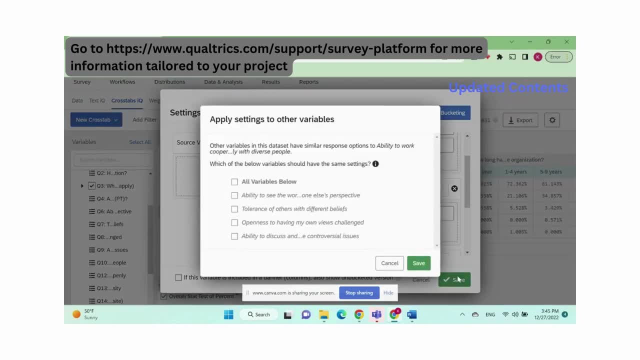 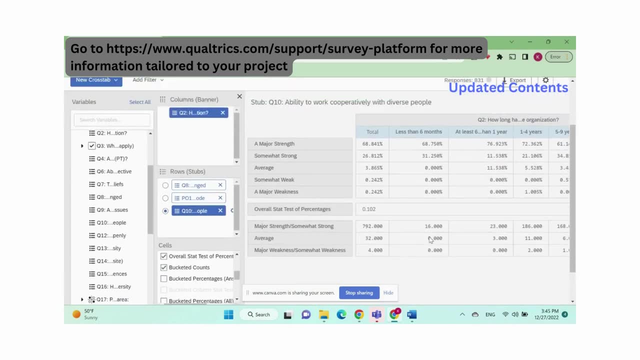 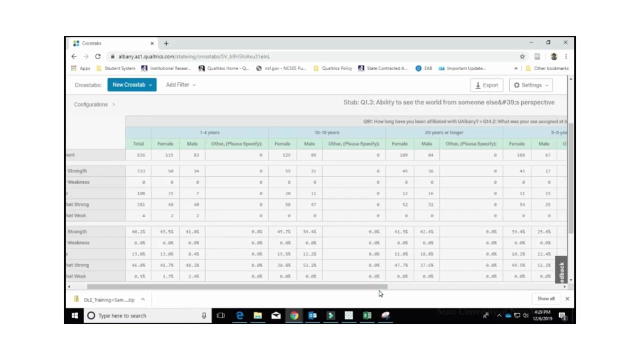 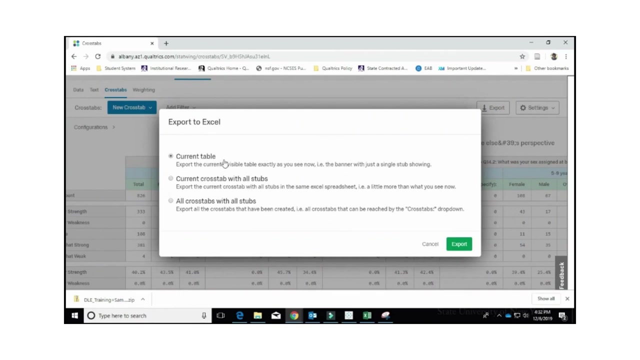 It is equal to the side. Thank you. There are two ways to export the crosstab results. You can select Export and then send all the tables onto an Excel sheet, Or you can hide the configuration sidebar. right-click and select Print to save the table in a PDF format. Thank you. 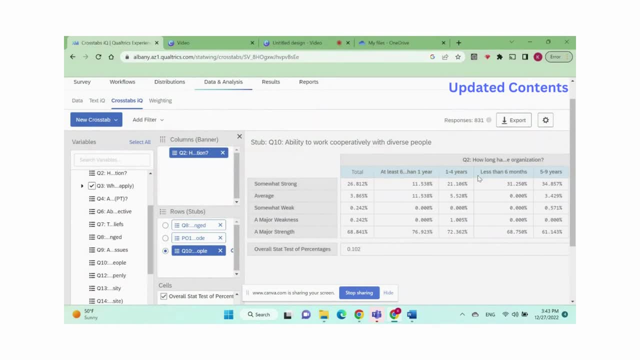 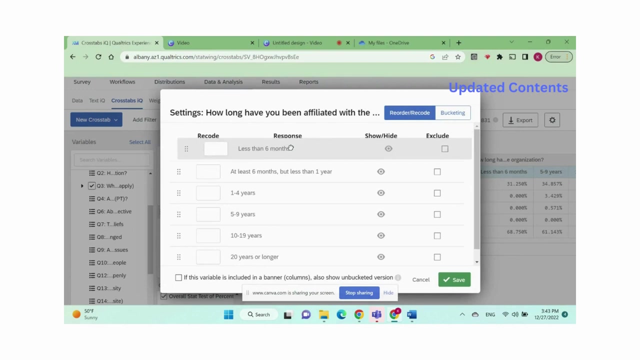 For example, in Question 2, less than six months option should be presented first before the choice at least six months, but less than one year. To reorder the choices, we click the setting icon of the variable in the banner window. Choose the choice you want to move and drag it to the right place. 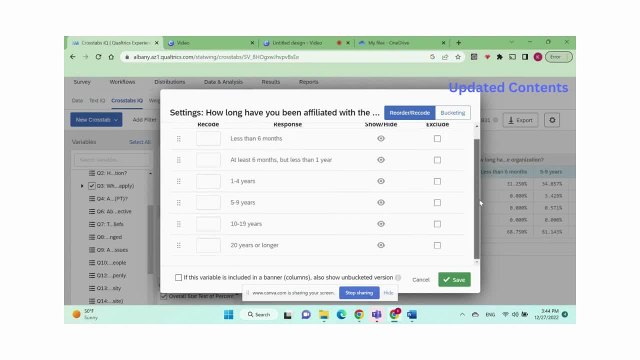 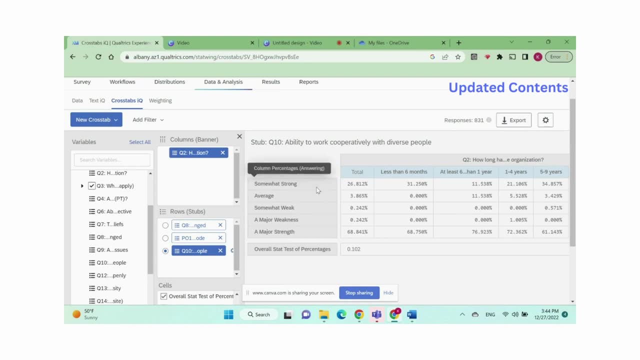 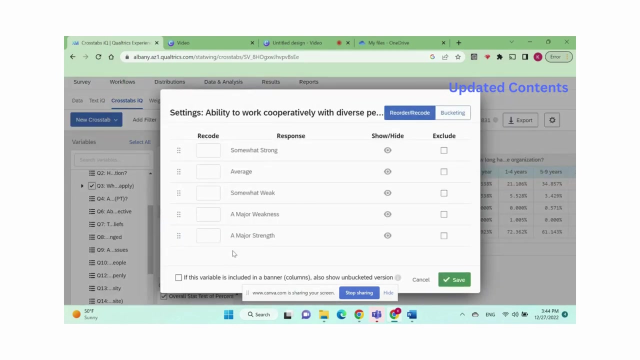 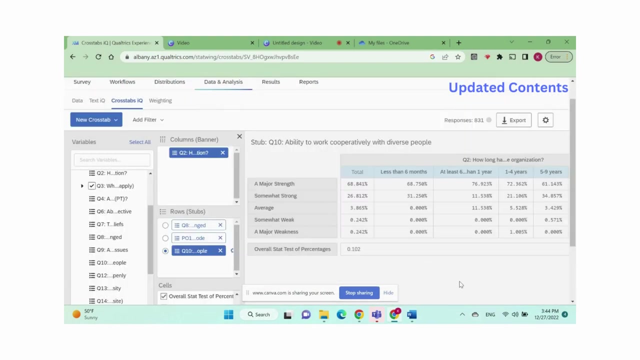 Then click Save. Same issue is found with the scale points in the rows. We click the setting icon of the scale variable in the stubs window, Drag the selected scale point to the correct place, Then save. Sometimes we may want to group some scale points together. 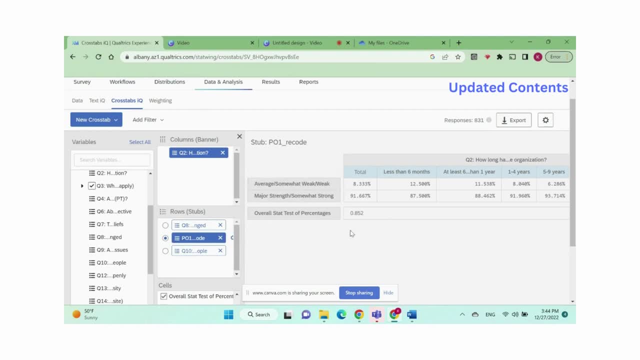 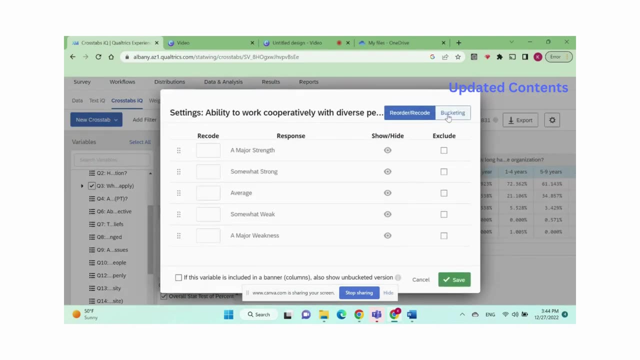 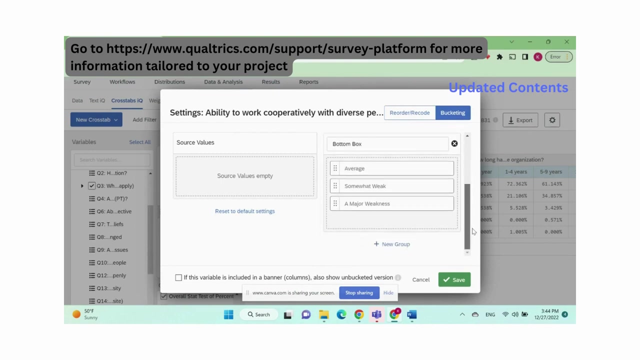 to get more meaningful analysis. For example, we can combine major strength in somewhat strong and major weakness in somewhat weak Together by using the bucketing feature in Qualtrics. You can also use some high and low strength values to get more meaningful analysis. 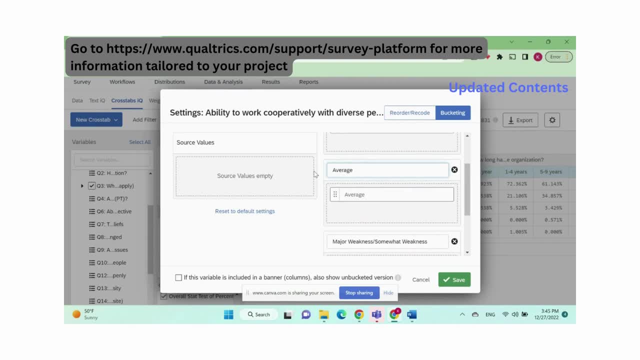 In this example we use the two-dimensional assessment of the scale and the scale. The scale and the scale-weight are ensure the same angle for the same measure of measurement. One more example: Let's have a look at the scale and the scale-weight. 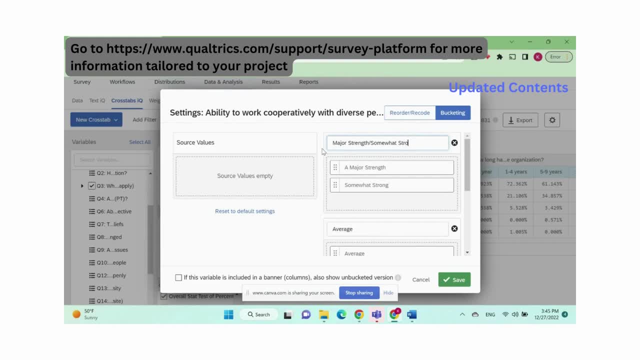 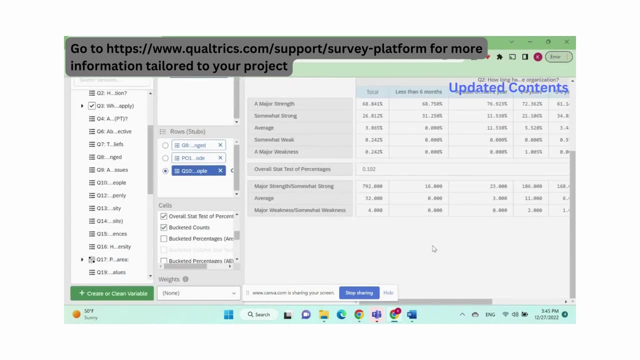 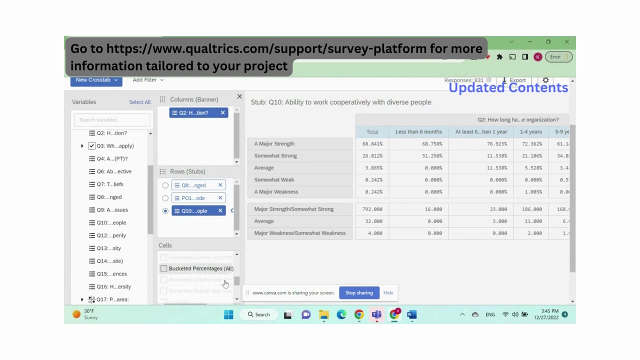 and see if you can see that they match up well with each other. Double-edged scale and scale-weight, So we can compare the size and the height of the scale. Thank you, There are two ways to export the crosstab results.